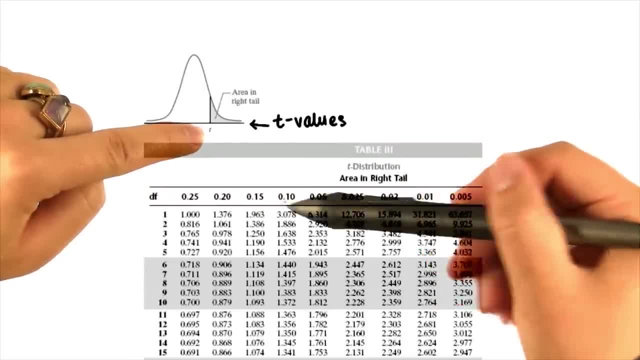 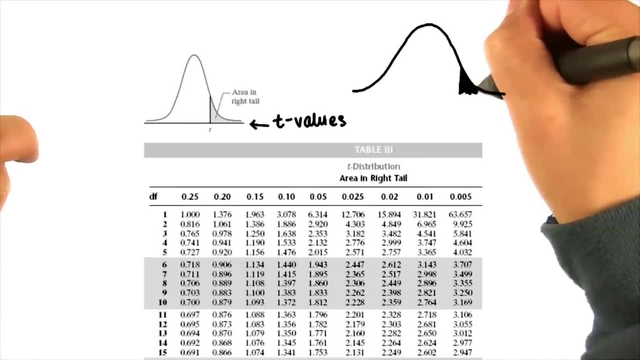 this case we only really care about the t-critical values. So let's say we have a t-distribution and we want to know the t-critical value, such that 10% is in the tail here, or a proportion of 0.1. And let's say that our sample size is 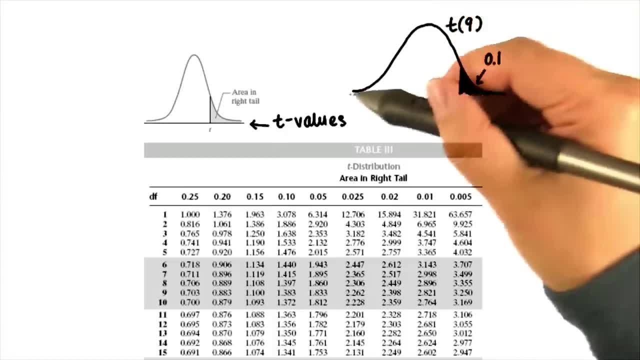 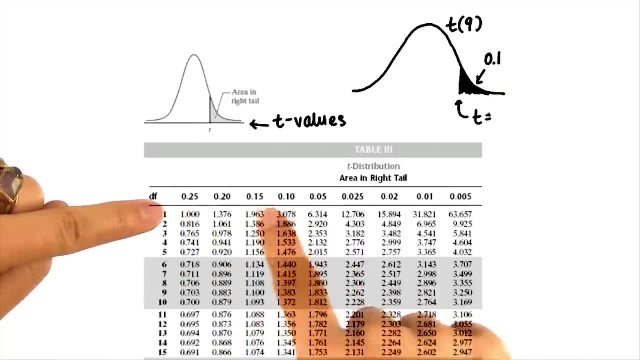 10,, so our degrees of freedom is 9.. So this is a t-distribution with 9 degrees of freedom, And we want to find this t-critical value. Well, here in the tails we look for 0.1.. And with 9 degrees of freedom, we see that the t-critical value is 1.383.. 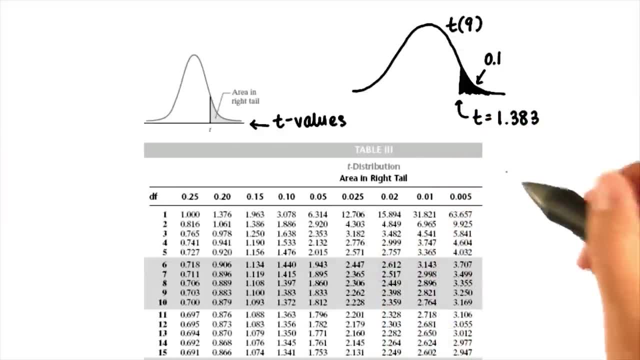 You're going to use this t-table to do pretty much the exact same thing you did with a z-table, But instead of finding the z-score and then determining if that z-score is bigger or less than the z-critical value, we find the t-statistic. 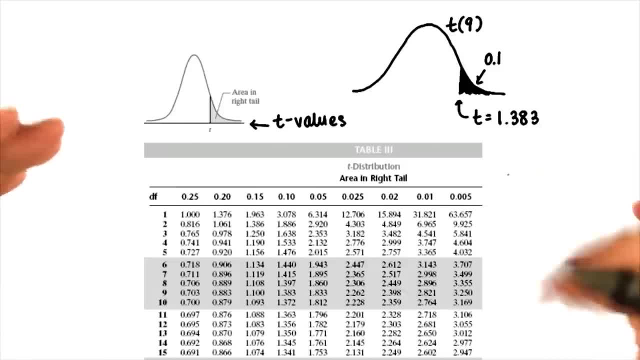 And we figure out if the t-statistic is greater or less than the t-critical value. Let's practice using the t-table.